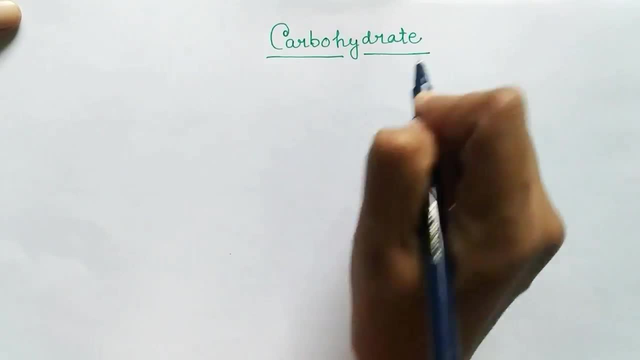 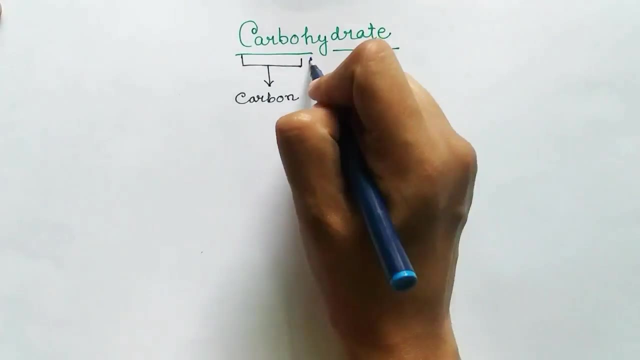 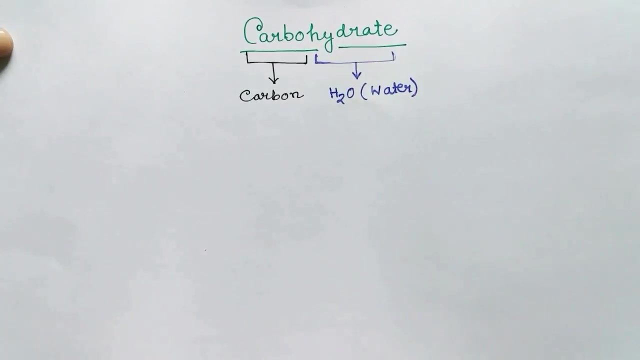 In this video we are talking about carbohydrates. So what do we mean by carbohydrate If we break the word? carbo means carbon hydrate, means H2O or water molecules, So carbohydrate means which is having carbon, oxygen and hydrogen. The molecular formula of a simple sugar is CnH2nOn, which can 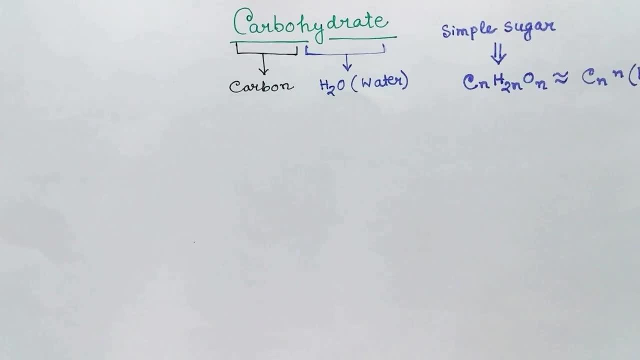 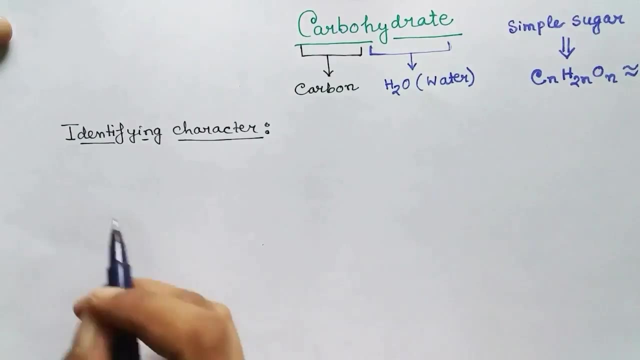 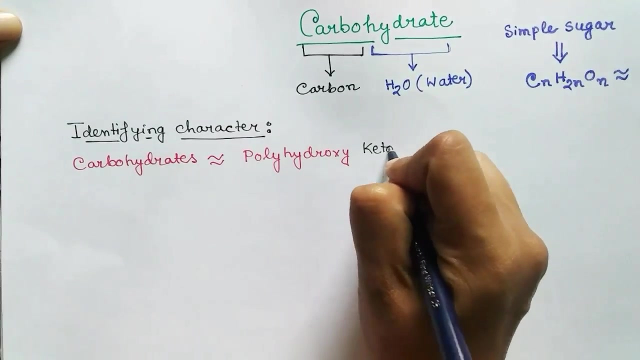 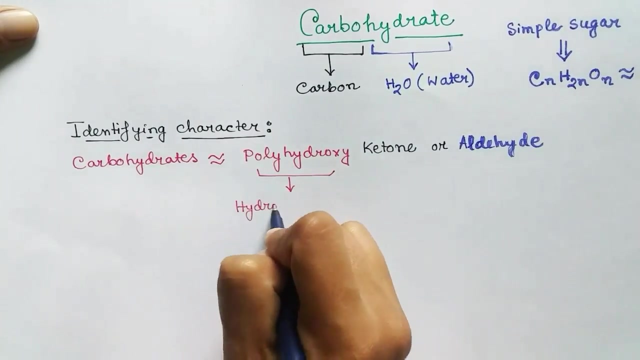 also be said as n number of carbon and n number of H2O. Now let's find out the identifying characters of a simple sugar. That means when can we call a molecule a sugar? Carbohydrate is a polyhydroxy ketone or aldehyde. Polyhydroxy means it has many hydroxyl group, which is OH group. 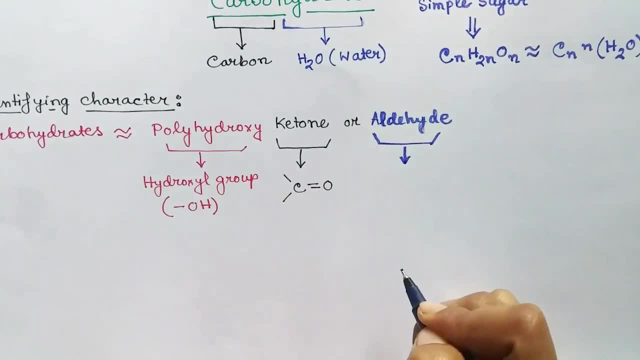 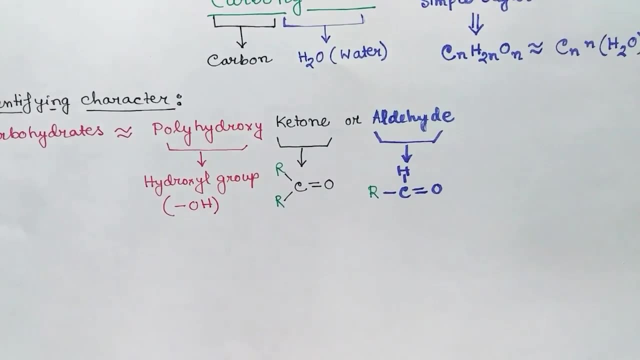 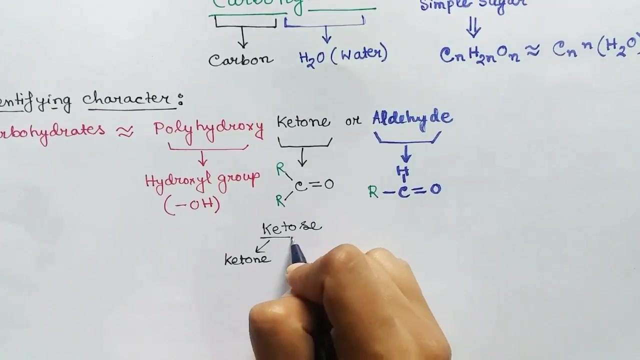 And it will have either one ketone group or one aldehyde group. So if we see a molecule with ketone or aldehyde group and having many hydroxyl groups, we can say that it is a sugar. The sugar molecule having ketone group is called ketose and the sugar molecule having an aldehyde 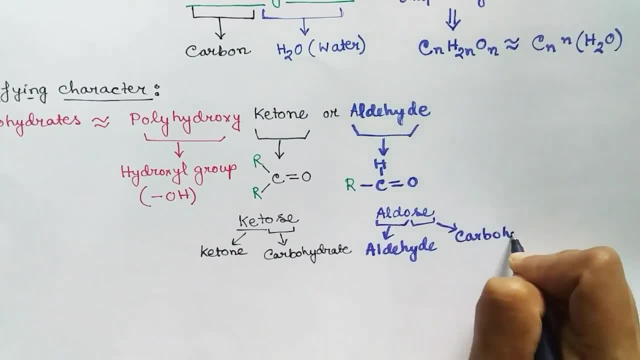 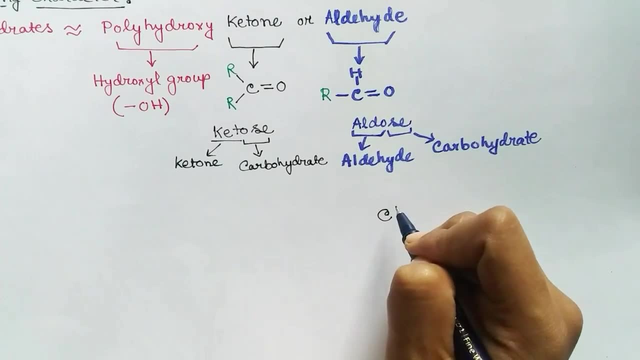 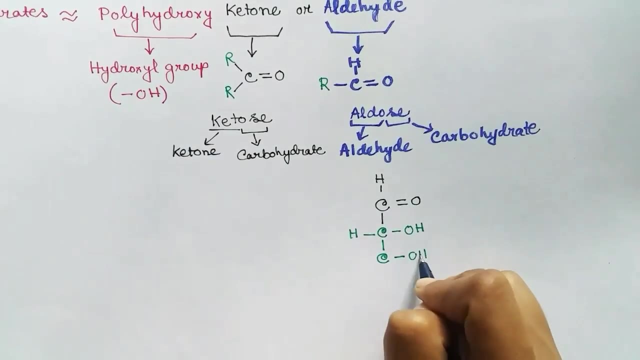 group is called aldose. Ose means carbohydrate. Now let's make a sugar, One sugar by ketone group and another sugar by aldehyde group. So this sugar, we have taken one aldehyde group and we have to take polyhydroxyl groups. So we have taken 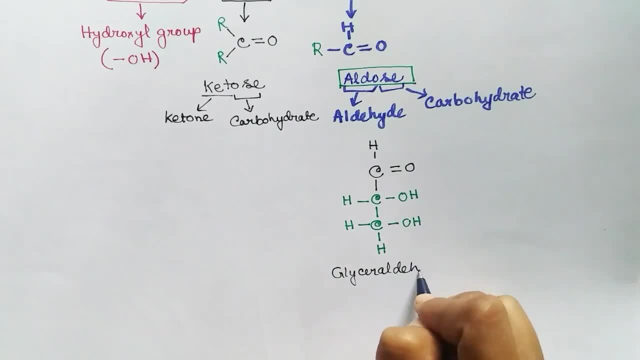 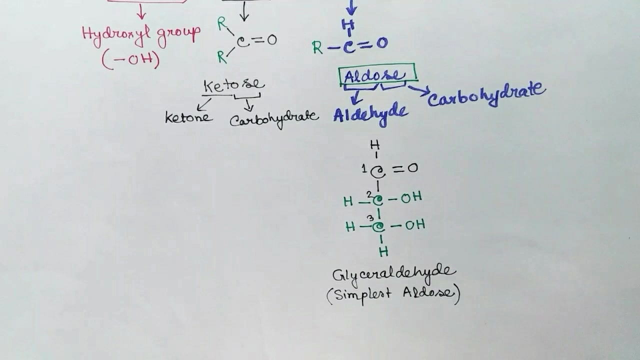 two hydroxyl groups. So this sugar is an aldose and it has aldehyde group And the name of this sugar is glyceraldehyde. and this is the simplest aldose. Simplest sugar molecule has at least three carbon atoms, Because if we remove the third carbon from 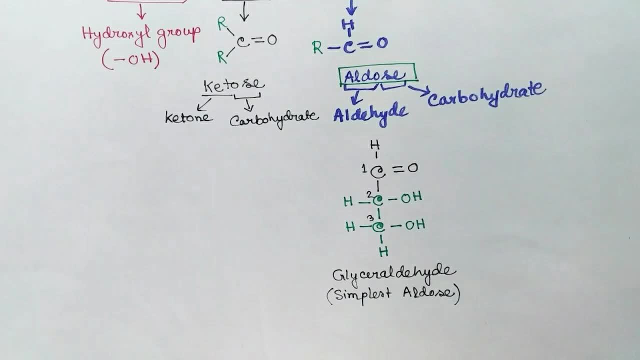 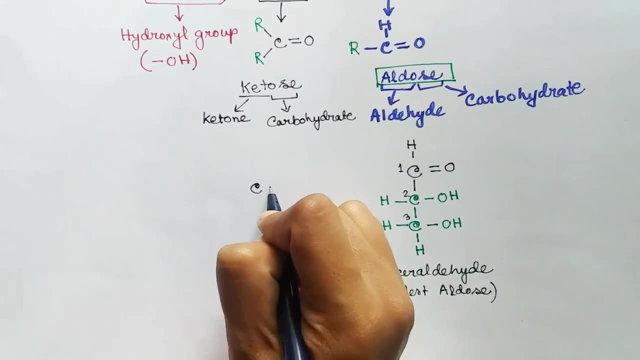 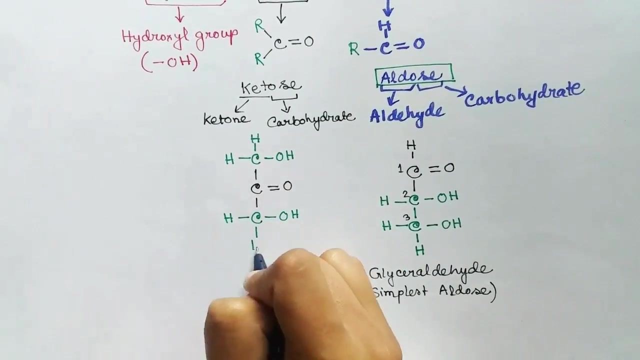 this molecule. we will not have polyhydroxyl group in this molecule, So we can only call it a sugar if it has polyhydroxyl molecules. Now let's make a sugar with one ketone group. So we have taken one ketone group and added two hydroxyl groups in another. 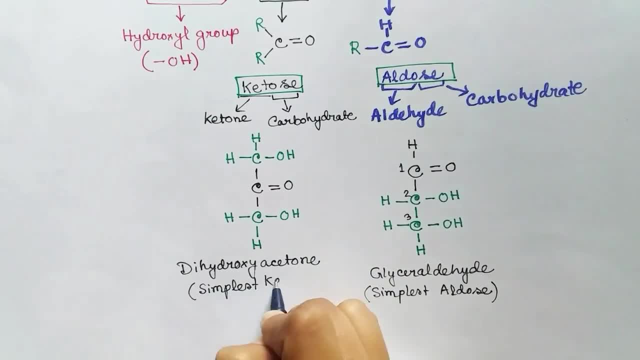 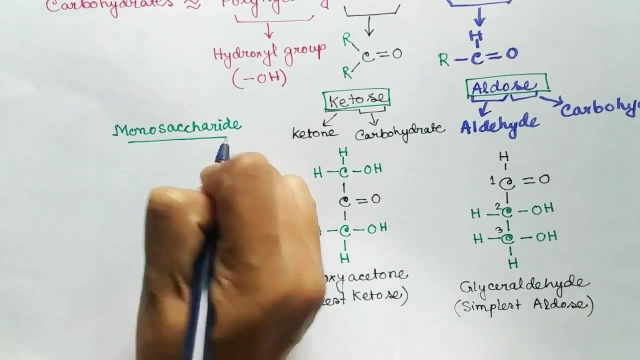 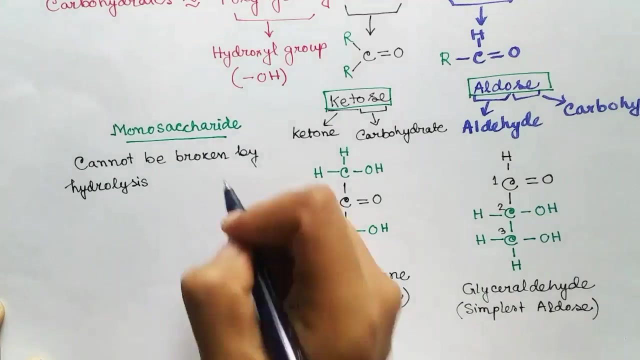 So this is the simplest ketose and the name of this is dihydroxyacetone. Each of the sugar is monosaccharide. Monosaccharide means the saccharide or sugar that cannot be broken by hydrolysis to make another sugar. So here you can see in both the molecules that if we hydrolyze the ketone or aldehyde group, then it will no longer remain a sugar, So we cannot break it into another sugar. Thats why they are monosaccharides. The simplest monosaccharide has three carbons in it, Thus called triose Monosaccharide, having four 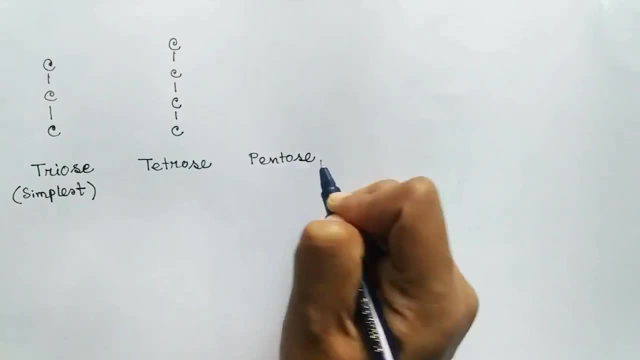 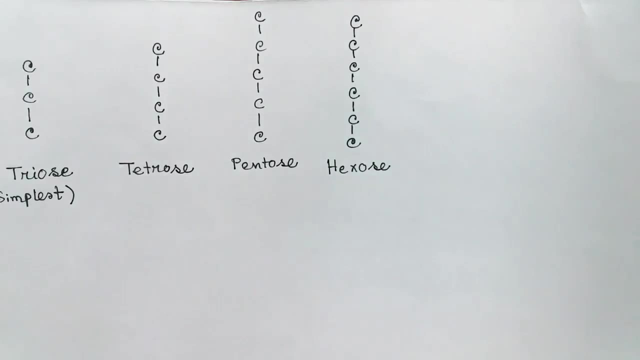 carbon is called tetrose. It has four carbon in it. Five carbon monosaccharides are called pentose. six carbon monosaccharides are called hexose, having six carbons in it. Seven carbon monosaccharides are called heptose and so 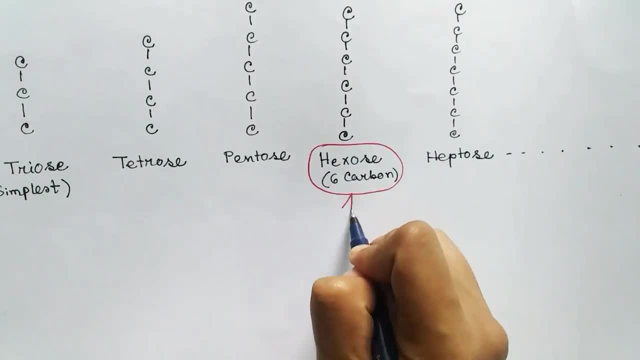 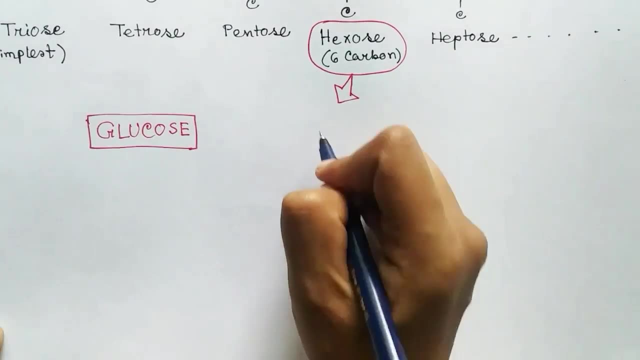 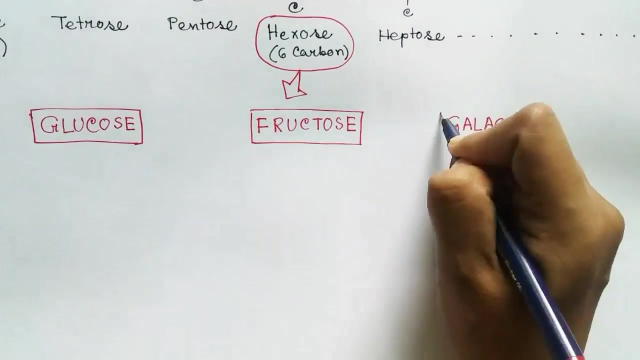 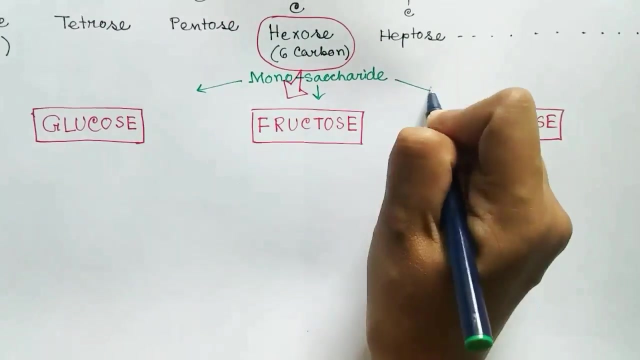 on. Here we will specifically focus on hexose, because some of the hexose monosaccharides are part of our food. The most well-known monosaccharides are glucose, fructose and galactose, and these are found in our food. All of these are monosaccharides and here we will see the 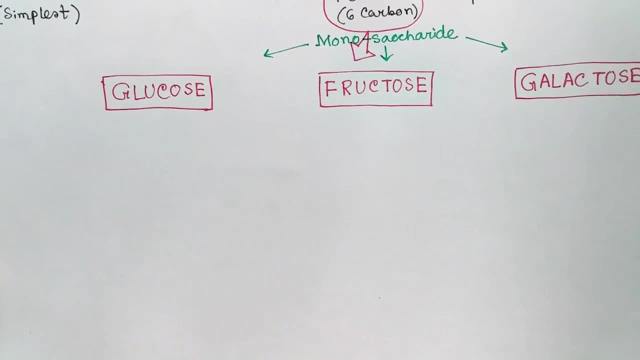 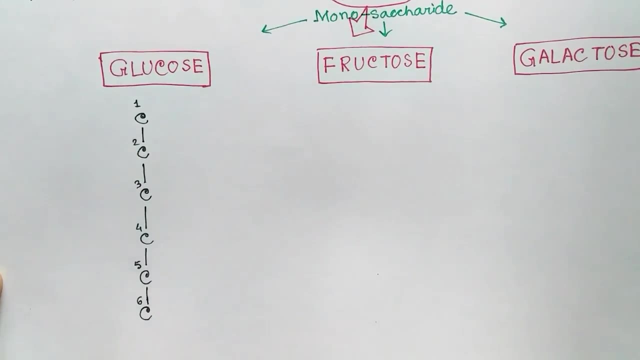 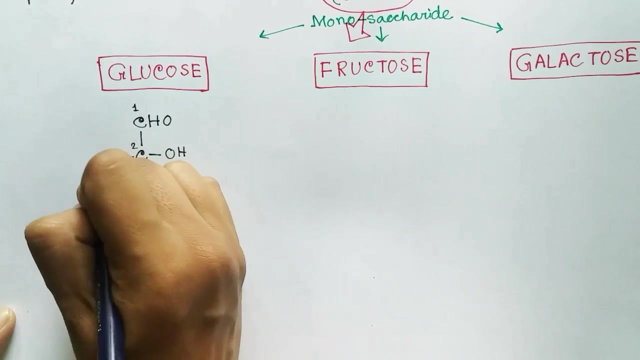 structures of each glucose, fructose and galactose. So let's begin with glucose. It has six carbon molecules To easily draw the glucose linear structure. I always remember these things. First, the first carbon will have the aldehyde group, The hydroxyl group on. the second carbon will 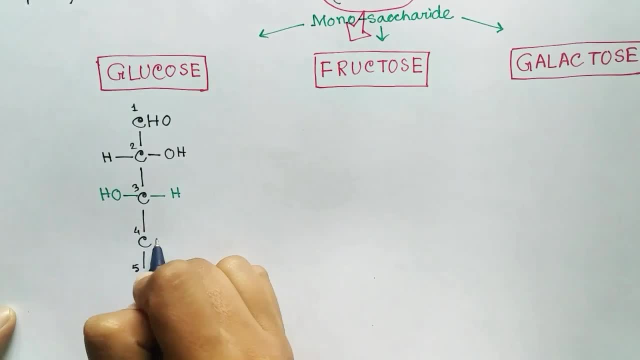 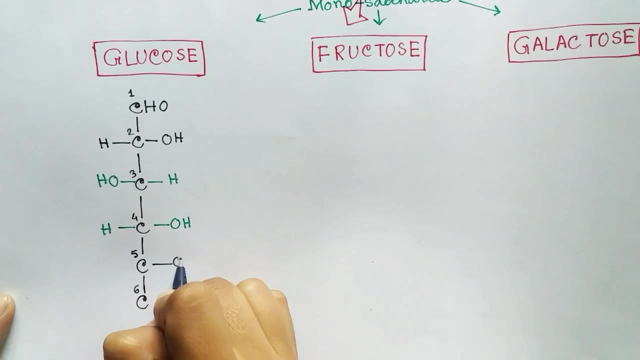 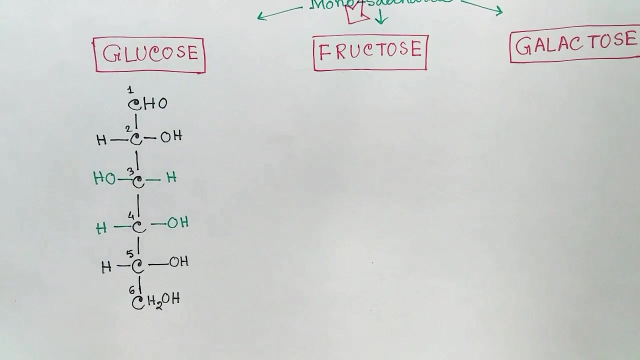 be on the right side and the third and fourth carbon hydroxyl groups will be in the opposite directions. The position of the hydroxyl group on fifth carbon depends on other factors, So we will discuss that later. So for now I am keeping it on the right side and the 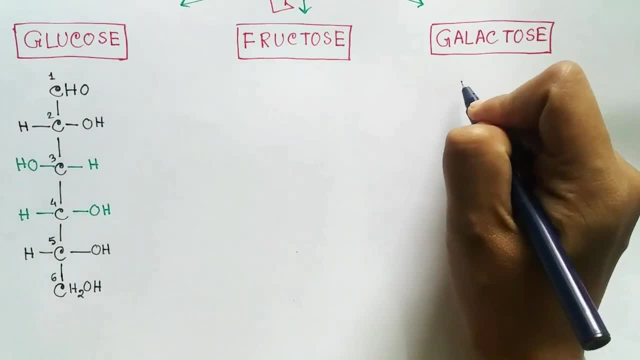 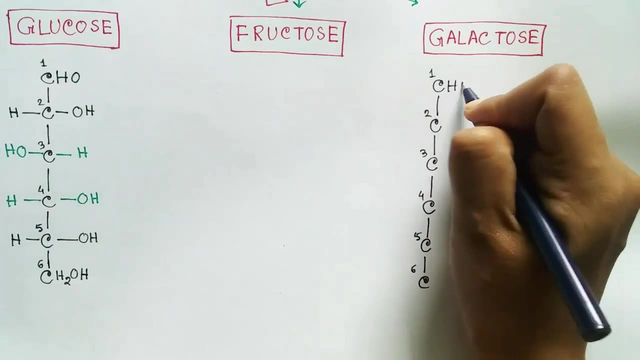 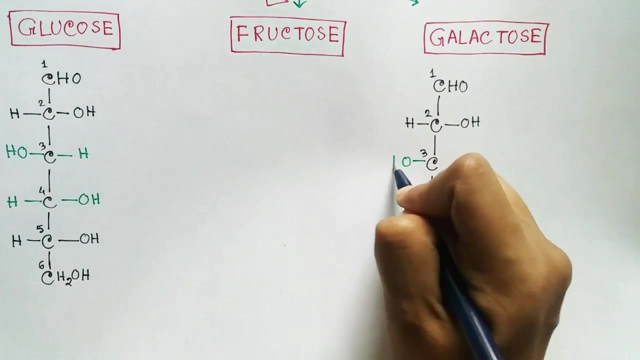 sixth carbon will have CH2OH. For galactose it is quite similar to glucose, Same as glucose. the galactose will have first carbon with aldehyde group, Second carbon with a hydroxyl group on the right side. but in case of third and fourth carbon, the 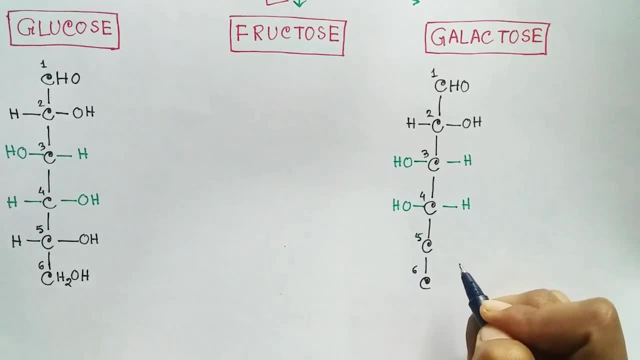 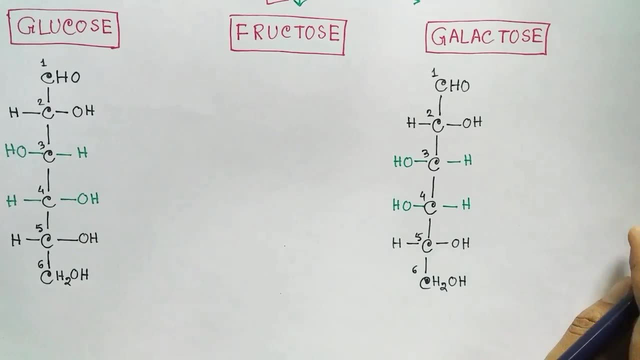 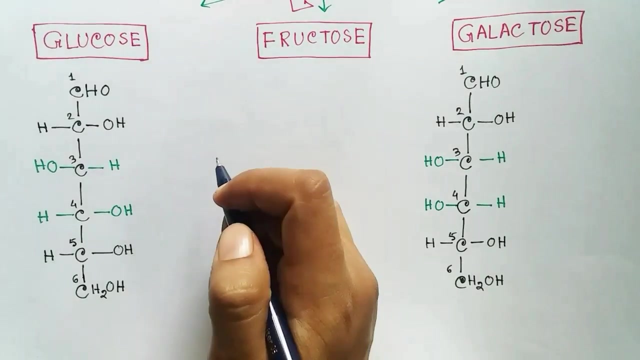 hydroxyl groups will be in the same side, which is not the case in glucose. So this is the only difference between glucose and galactose structure. So the third and fourth carbon will have hydroxyl group on the same side. Now let's draw the fructose. The fructose is a ketose. that means it. 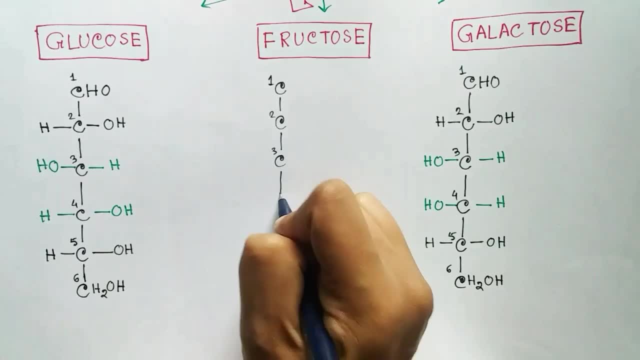 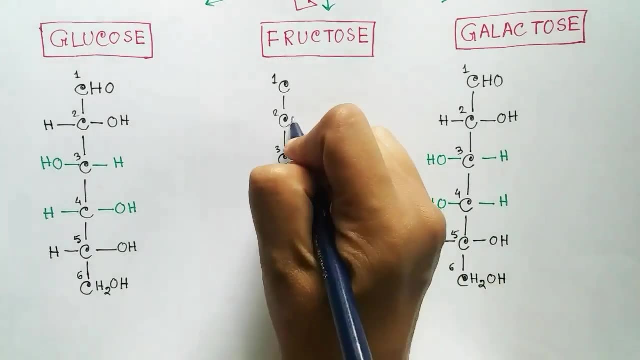 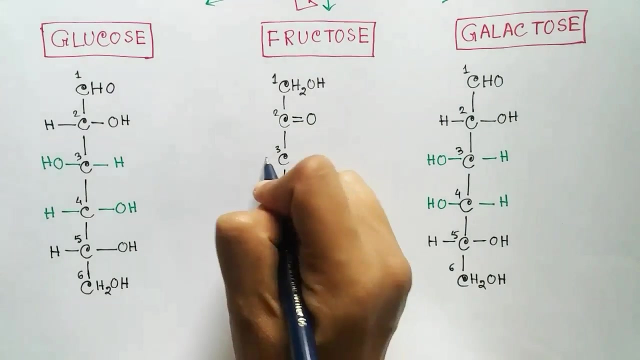 has a ketone group, not an aldehyde group, In the fructose structure. everything is quite similar to the glucose structure, except the ketone group. So the ketone group of the fructose is present in the second carbon, and the first carbon will have CH2OH and the third and fourth carbon will be 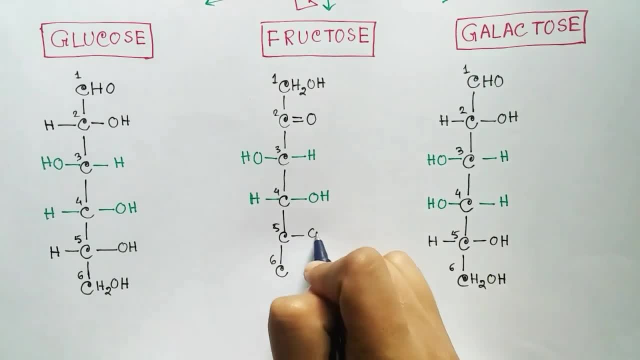 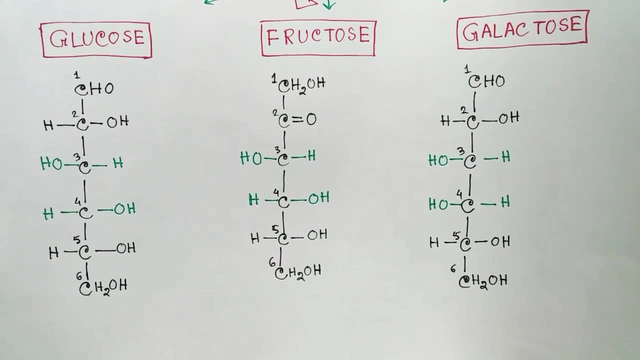 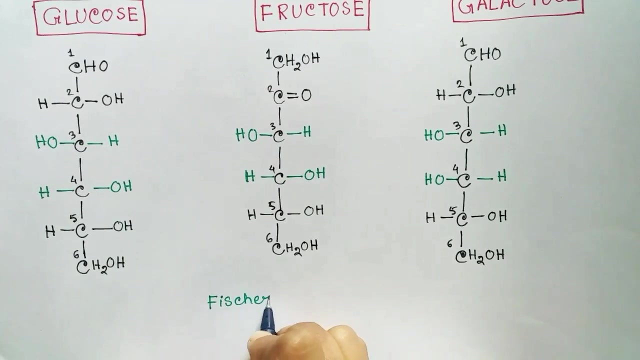 similar to glucose, that is, the hydroxyl groups are present in opposite and the fifth and sixth carbon will be similar to the glucose structure. So the only difference is the ketone group in fructose. All these structures that I have drawn are linear structures. These kind of linear 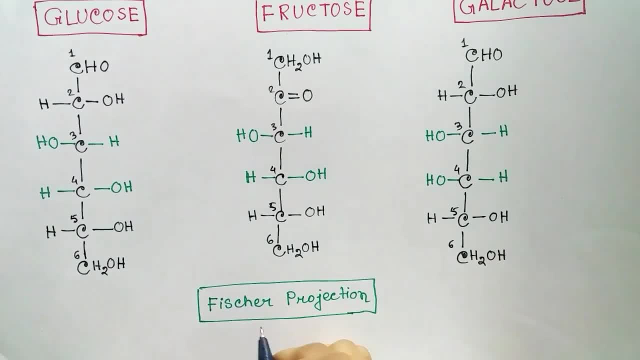 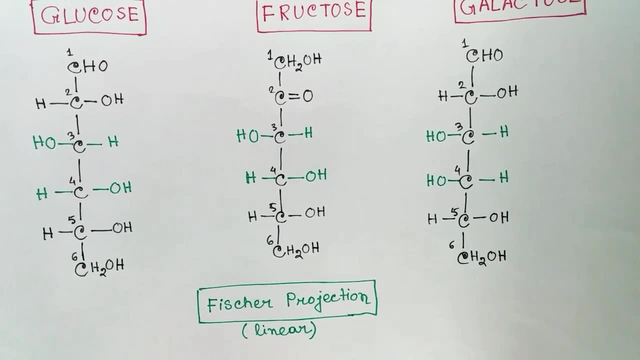 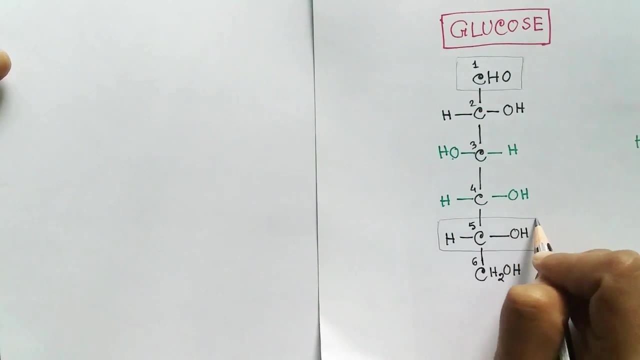 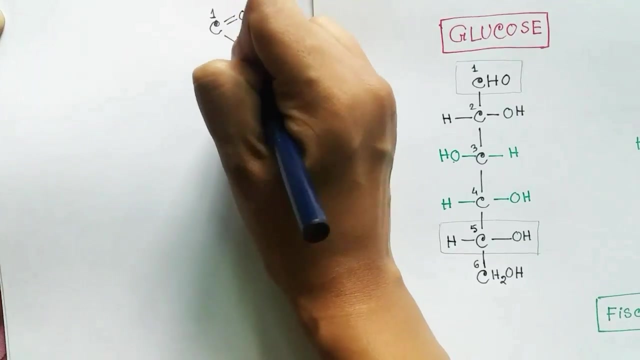 structures are called Fischer projections, but only two to three percent of these molecules remain in the linear structure. These molecules, such as glucose, fructose and galactose. they usually remain in the cyclic form. So let us see how the cyclic form is formed and how it looks In the cyclic form of glucose. the 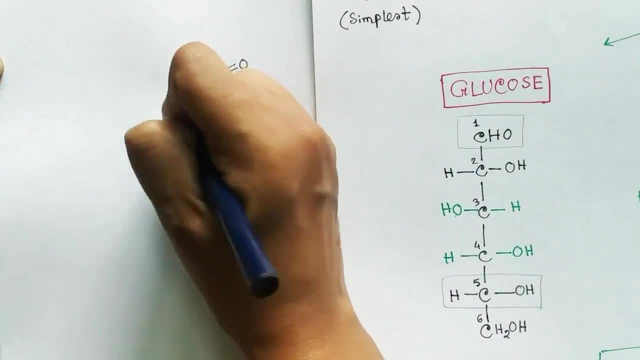 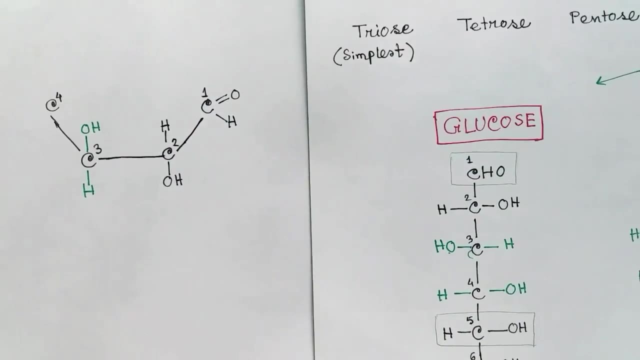 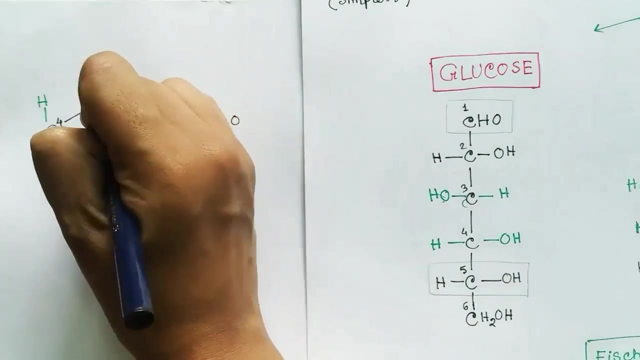 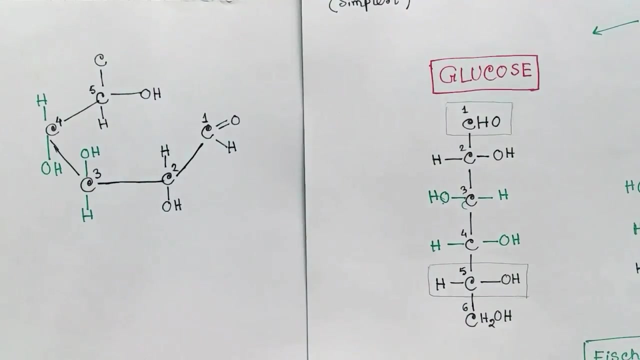 aldehyde group reacts with the hydroxyl group of the fifth carbon to make a stable structure. So let us bend the linear structure of glucose and bring the fifth carbon hydroxyl group near the aldehyde group of the first carbon And the sixth carbon. CH2OH remain either above or below the plane of the cycle. So the fifth carbon 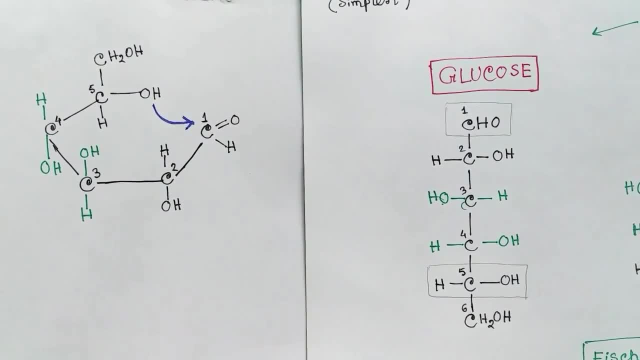 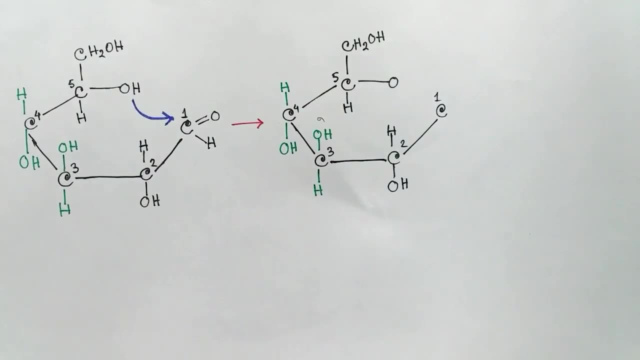 hydroxyl group will react with the aldehyde group of the first carbon. This reaction is called hemiacetal formation. By this reaction, or the formation of the bond, the first carbon will have one hydroxyl group, either above the plane or below the plane of the cycle. 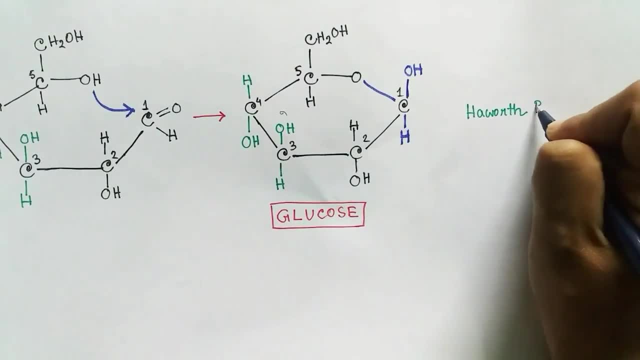 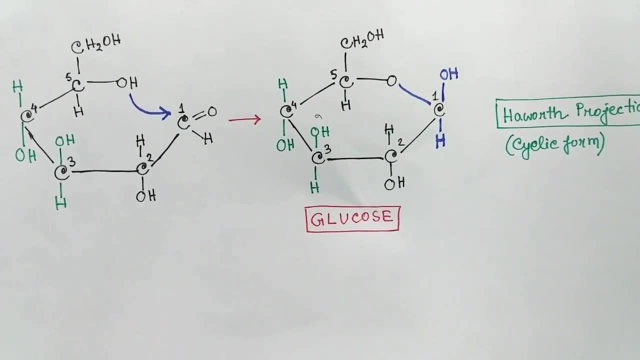 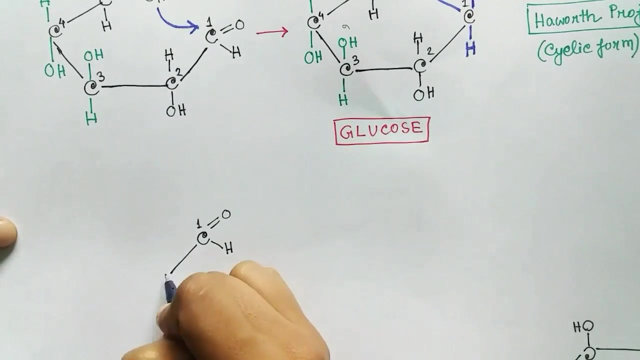 So this is the cyclic structure of glucose. This kind of cyclic structures are also called Haworth projection: 97% of the glucose in a solution remain in the cyclic form, not in the linear form. Now coming to the cyclic form of the galactose, which is very much similar to the glucose, but 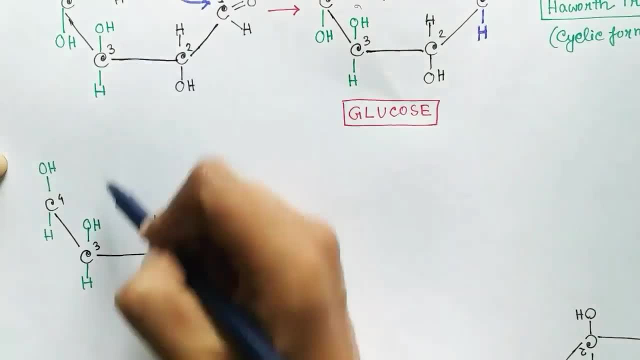 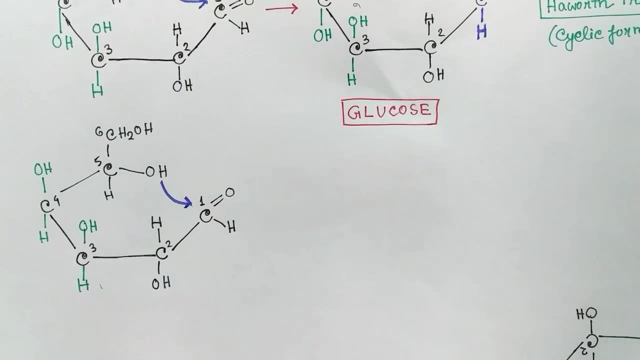 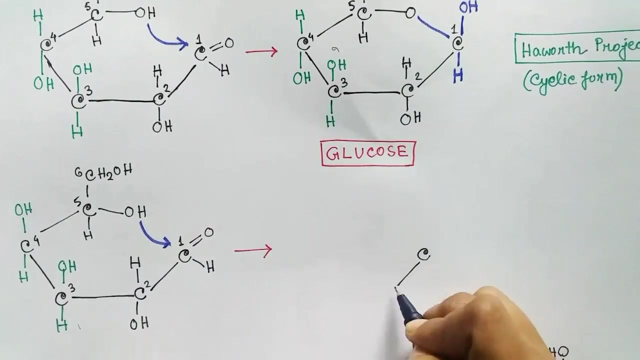 not in the third and the fourth carbon. In the third and the fourth carbon the galactose will have the hydroxyl groups on the same side. Otherwise the cyclic structure of galactose is quite similar to the glucose. So here the first carbon will also react with the hydroxyl group of 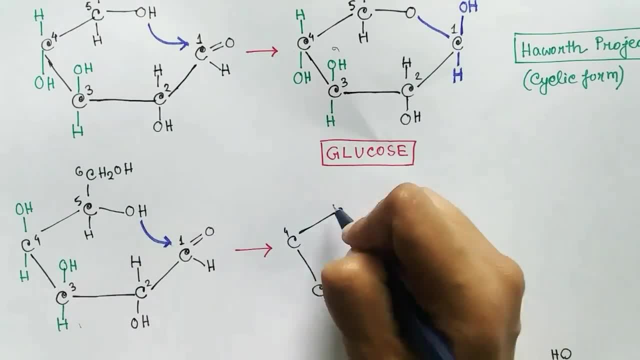 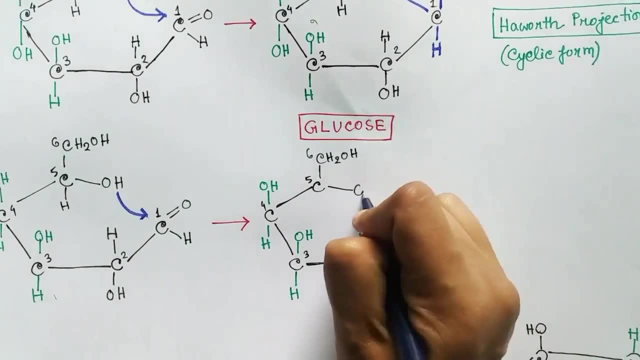 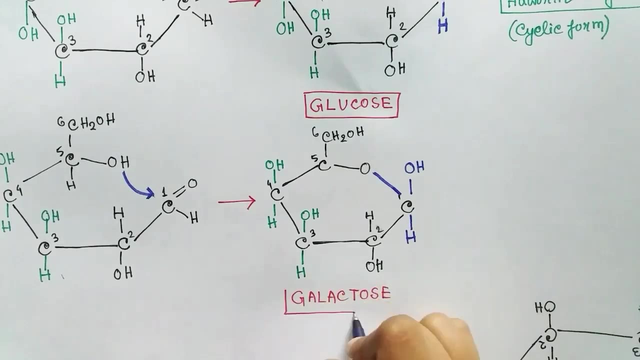 the fifth carbon for stability, and it will form the cyclic structure of the galactose. And this is also the hemiacetal formation, as this is also an aldose And the first carbon will have an hydroxyl group above or below the plane. So this is the galactose in cyclic form. 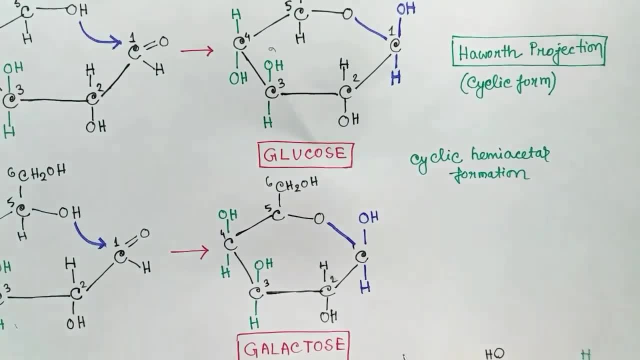 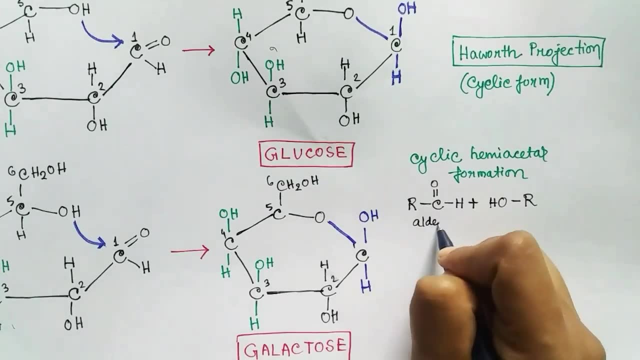 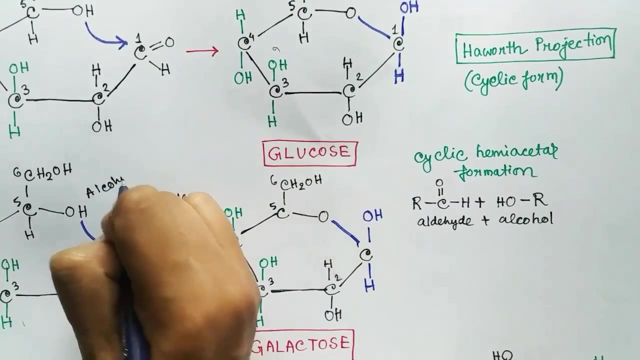 I mentioned the formation of hemiacetal in both the case of glucose and galactose. So let's see what is hemiacetal formation? Hemiacetal is when an aldehyde group reacts with alcoholic group. So this is the aldehyde group and this is the alcoholic group, that is the OH group. 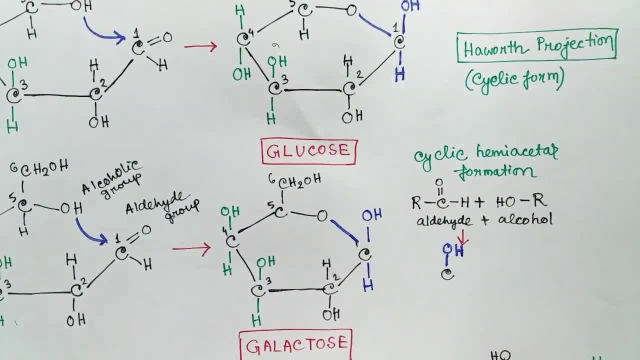 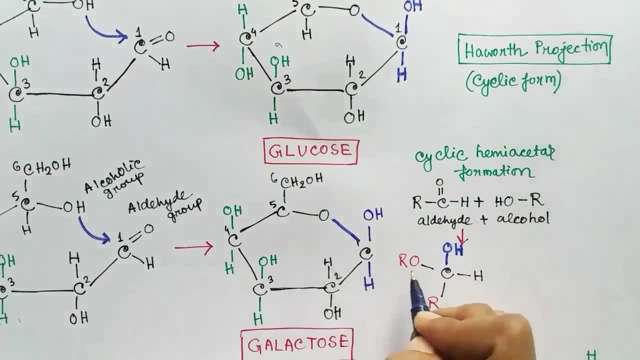 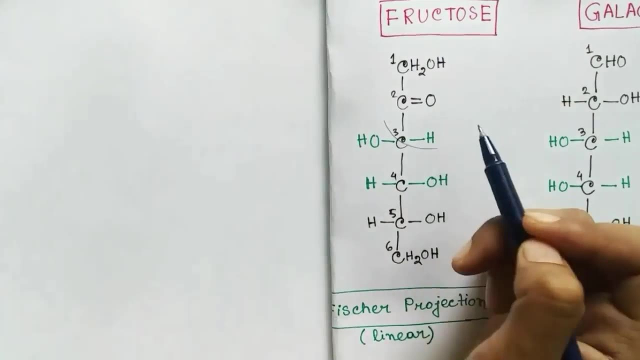 When they react, what it forms is the hemiacetal. The hemiacetal carbon will be the first carbon which was having the aldehyde group, and the hemiacetal looks something like this: Now let us see the cyclic form of the fructose. The fructose is a ketose. that means it is having a 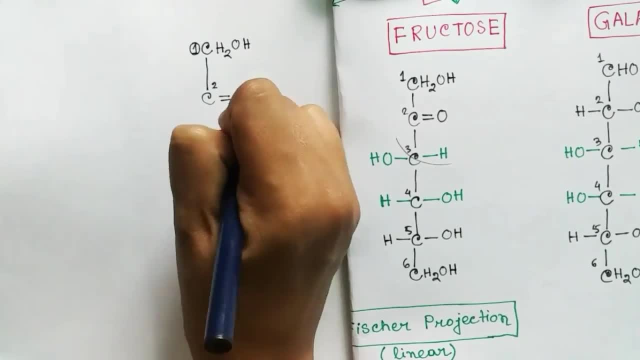 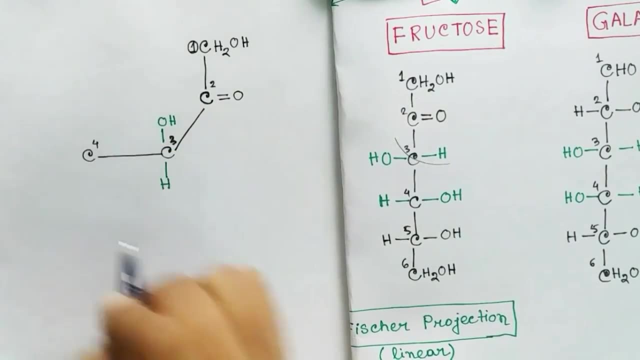 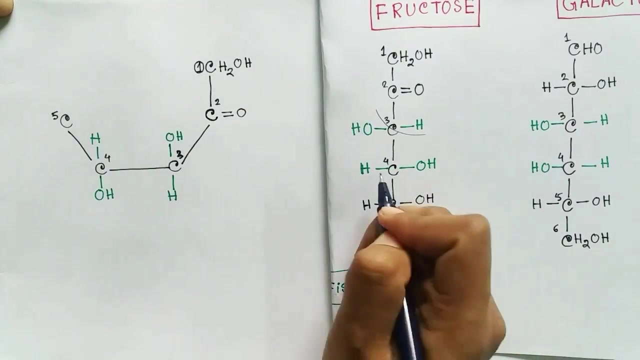 ketone group. So the reaction in the cycle will be quite different. from the glucose and galactose which are aldoses, Fructose, the functional group, the ketone group, is on the second carbon. so this time the second carbon will react with the hydroxyl group of another carbon. In case of fructose it can happen. 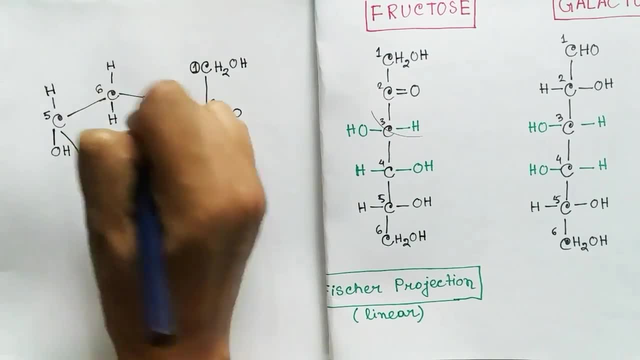 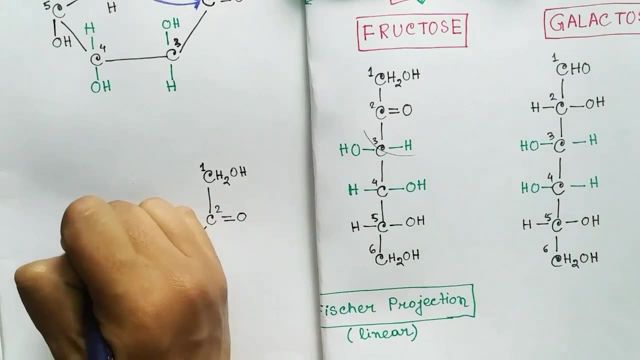 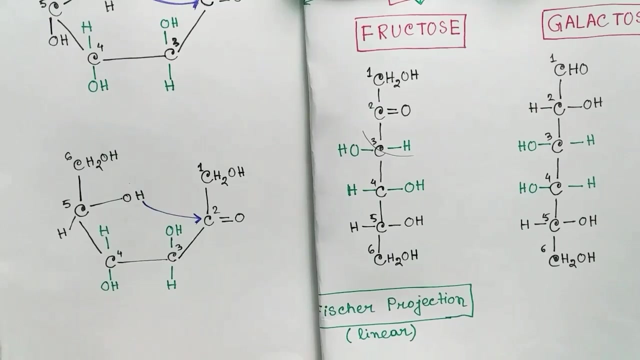 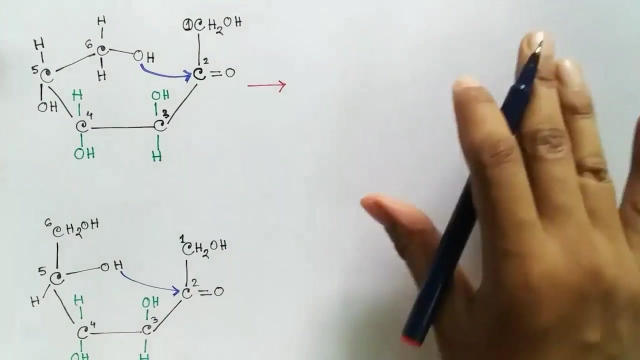 in two ways. The second carbon, the ketone carbon, can react with the hydroxyl group of the sixth carbon, or it can react with the hydroxyl group of the fifth carbon. Both the cyclic forms are stable in fructose In case of reaction with the hydroxyl group of sixth carbon, the cyclic form. 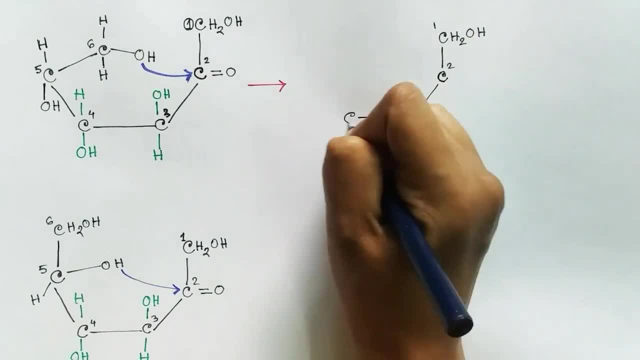 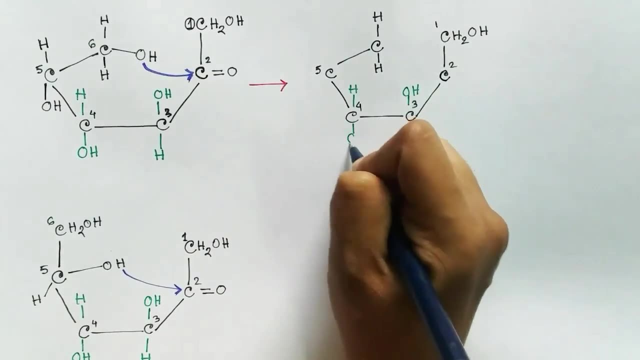 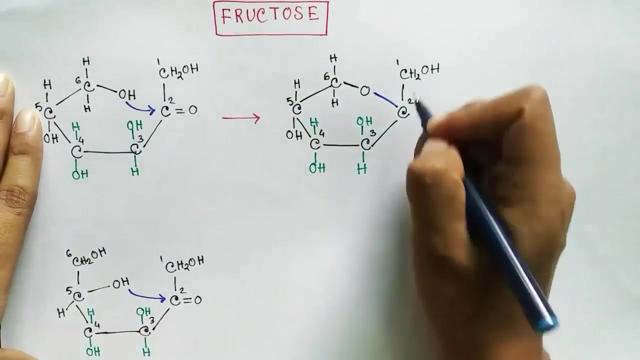 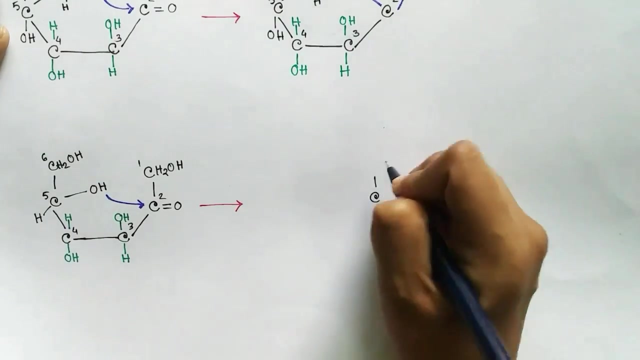 contains five carbon inside the ring. So this is the form when it reacts with the hydroxyl group of the sixth carbon. So it has five carbon inside the ring and the first carbon remain above or below the plane of the cycle. In case of reaction with the hydroxyl group of the fifth carbon, the ring contains four carbons and 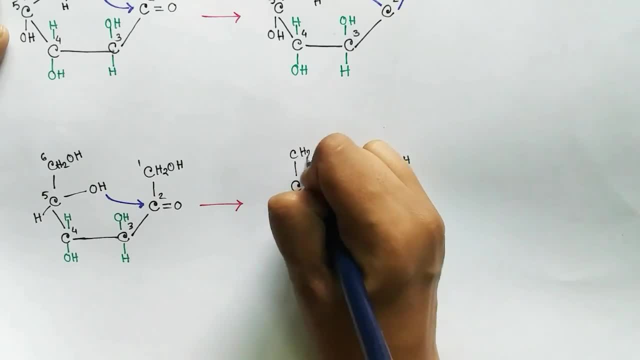 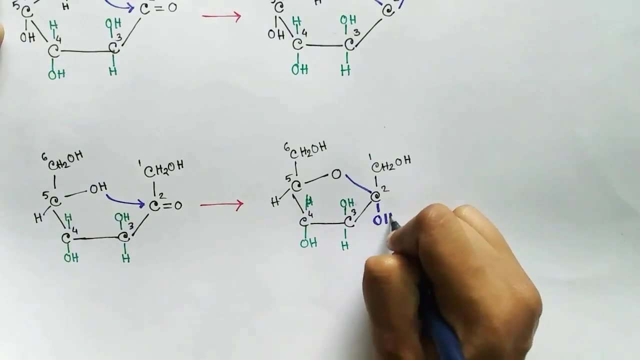 the first and the sixth carbon remain above or below the plane of the ring. So you can see here one CH2OH is above the second carbon and the other CH2OH is above the fifth carbon. Now this ring is called the pyranode. 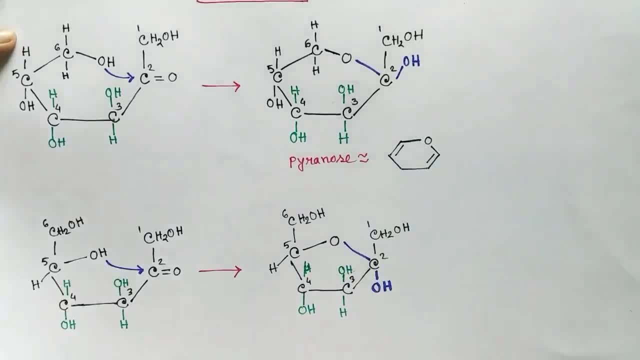 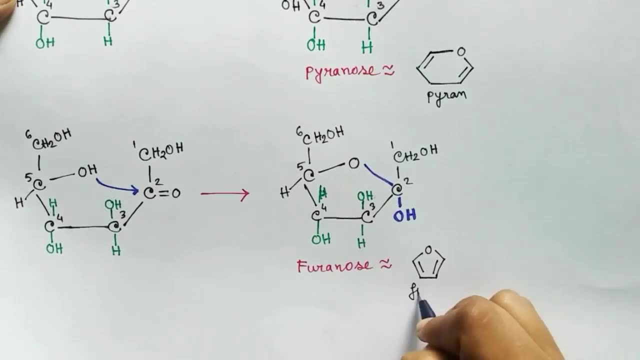 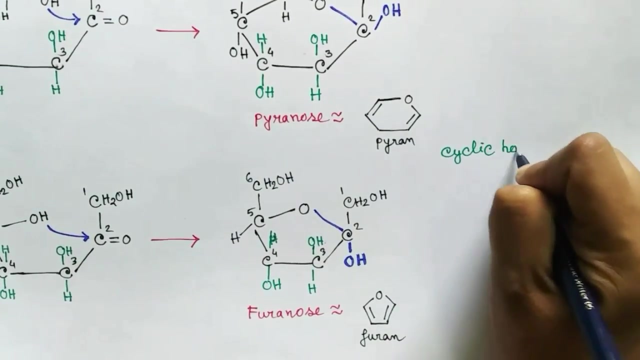 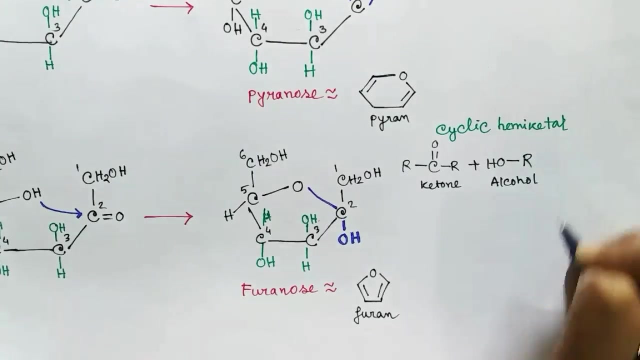 Because it is similar to the pyran ring and this ring is called the furanose because it is similar to the furan ring. In this case, the hemi-ketal formation occurs because the functional group of fructose is ketone. So what is hemi-ketal When a ketone group reacts with the alcoholic group? 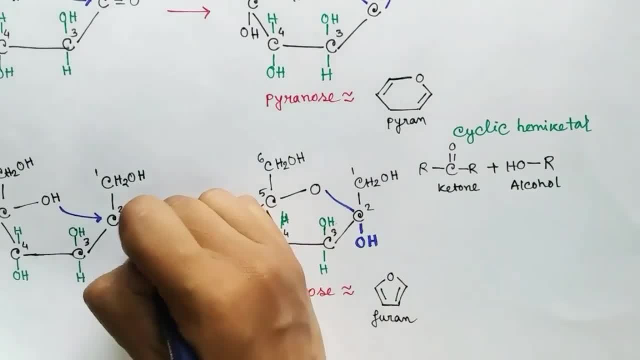 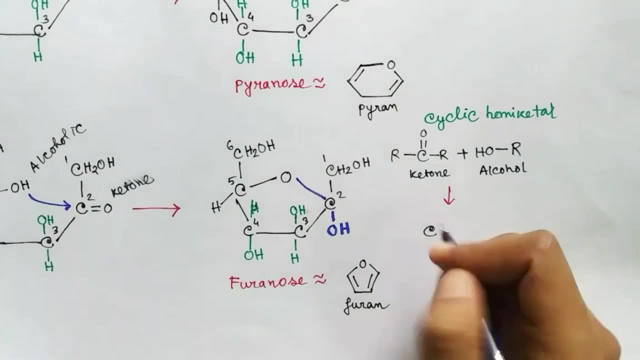 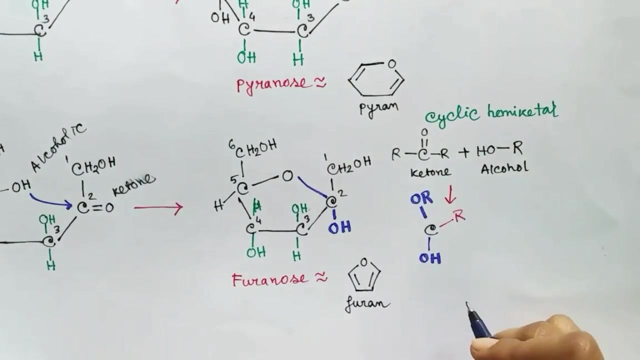 it forms hemi-ketal, So it is the ketone and it is the alcoholic group. When they are reacting, hemi-ketal formation occurs and the hemi-ketal carbon is the carbon which was carrying the ketone group. So the hemi-ketal looks something like this: 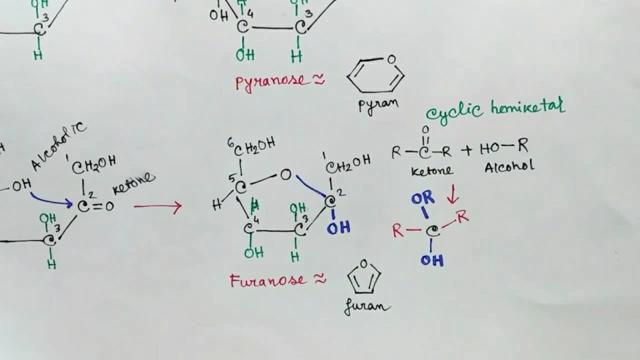 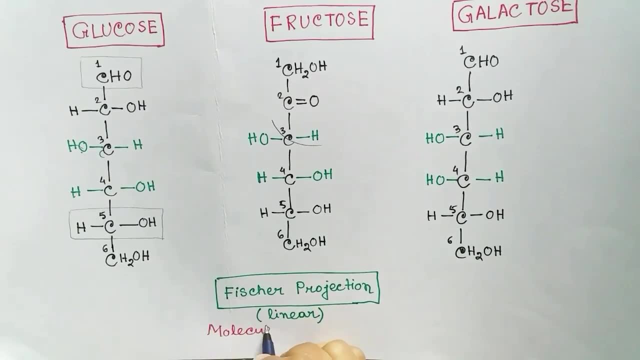 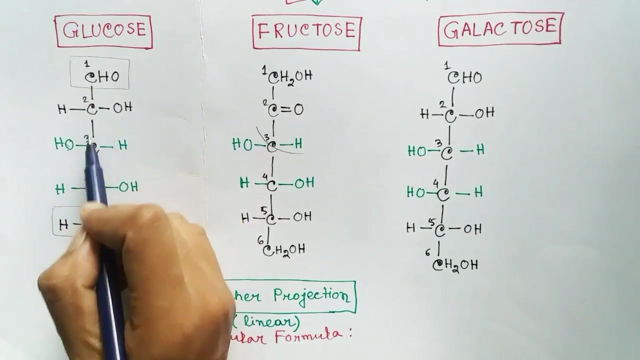 which is quite similar in the ring. Now let us look into the molecular formula of glucose, fructose and galactose, As they are all hexose, the number of carbon is 6 in all the cases, So the number of carbon in glucose is G6. 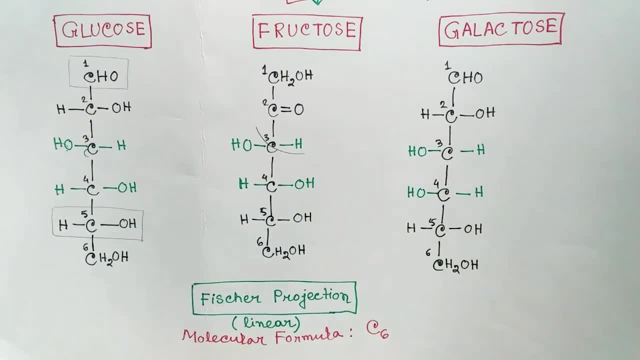 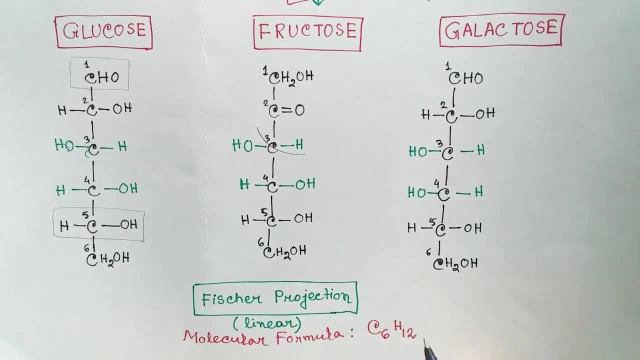 C6. And if you count the number of hydrogen it will be 12.. So the number of hydrogen is 12 and number of oxygen in glucose is 6.. So it's C6, H12 and O6. And if you count the carbon,